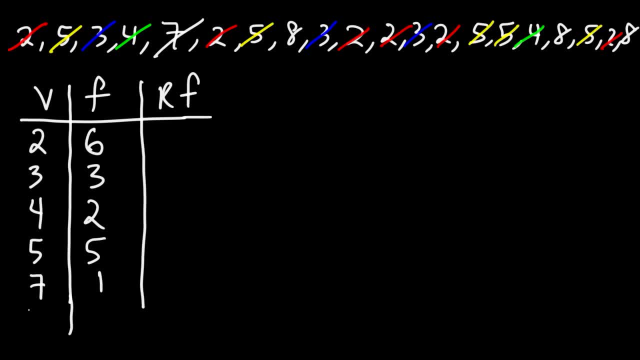 I only see one: 7.. And finally, the highest value is going to be 8.. And so there's 1,, 2,, 3, 8s. Our next step is to take the sum of the frequency column. 6 plus 3 is not a 3.. 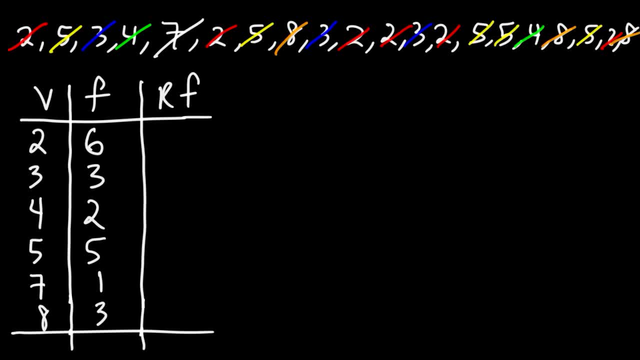 So we're going to take the sum of the frequency column: 6 plus 3 is not a 3. plus 2, that's 11, plus 5 is 16,, plus 1 is 17, and then plus 3 is 20.. Now to calculate the. 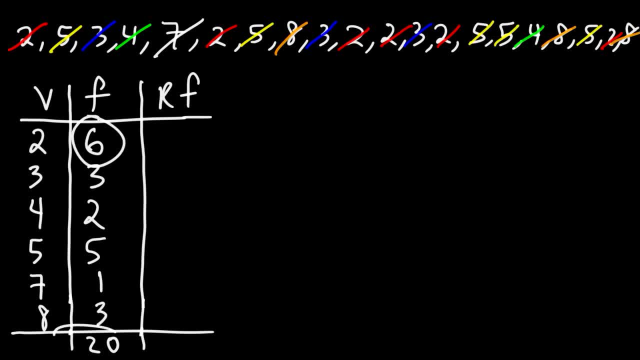 relative frequency. take the frequency and divide it by the total frequency, So 6 divided by 20.. If you type this in your calculator, you should get 0.30.. Next let's take 3 and divide it by 20.. 3 divided by 20 is 0.15, and then we're going to follow the 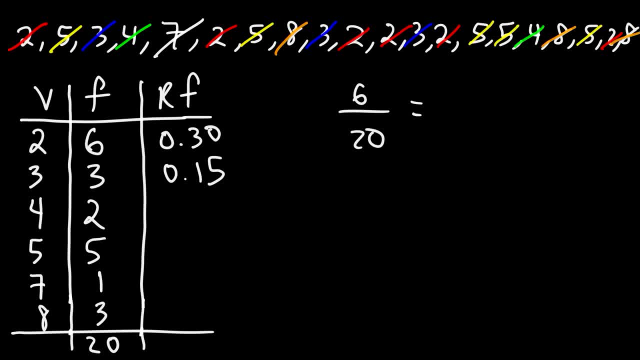 pattern. So now let's divide 2 by 20.. So this is going to give us 0.1, which is the same as 0.10, and then we're going to have 5 divided by 20,. 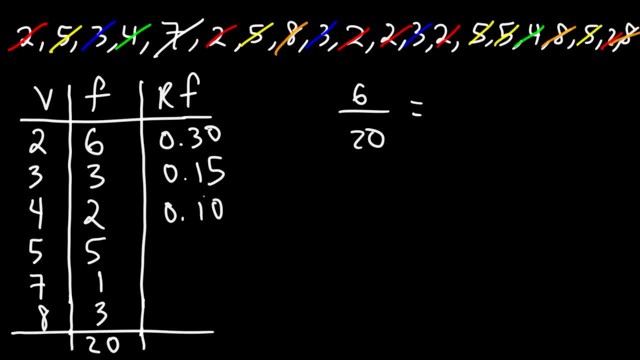 and so that's 0.10.. Then it's 1 divided by 20, which is 0.05, and here we have a 3 again. So we know 3 divided by 20 is 0.15.. So that's how we can obtain the relative. 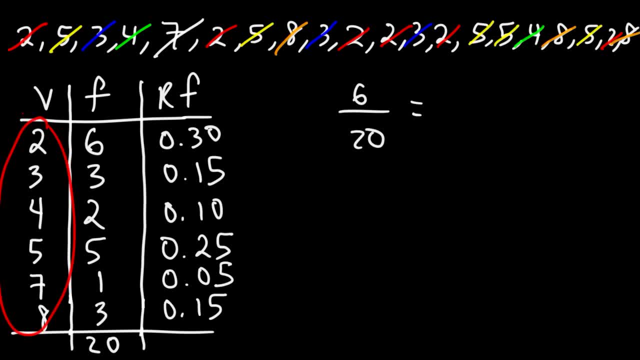 frequency for each of the values here. So the relative frequency for, let's say, a value of 4 would be 0.10.. The relative frequency for, let's say, 8 is 0.15.. Now here's how you can test to make sure that you did it correctly. Add up all the 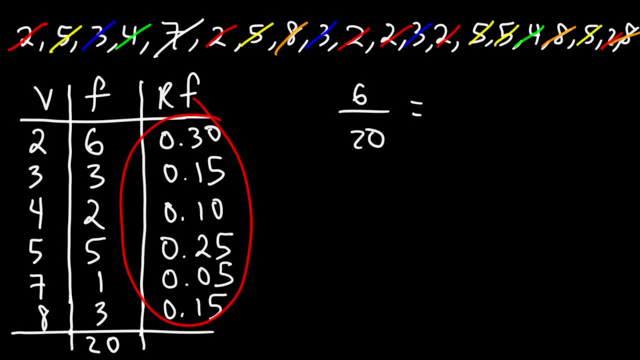 values of the relative frequency and you should get 1.0.. So if you take 0.3 and add it to 0.15, plus 0.10,, plus 0.25, plus 0.05, and then plus 0.15 again, you should get exactly.